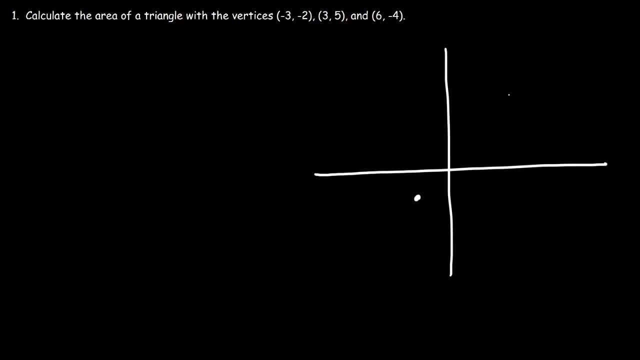 is just a ballpark estimate, And the second point is at, which is probably going to be somewhere over here, And the third one is at, which is probably going to be in that region, And so we have a triangle that looks roughly like this. So let's call this A, B and C. So A is at, B is at and C is at. 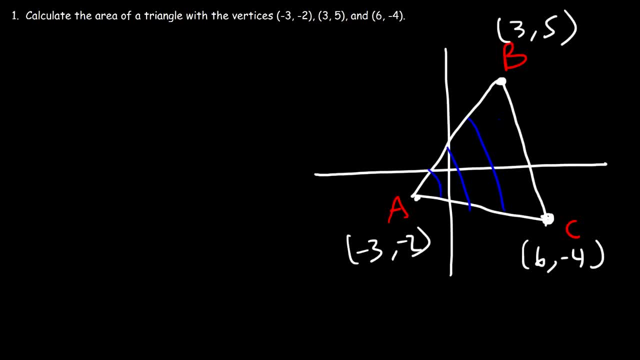 So how can we calculate the area of this triangle? So let's call this. So let's call this. So let's call this X1 and Y1.. This is going to be X2 and Y2, and this is X3 and Y3.. So I'm going to 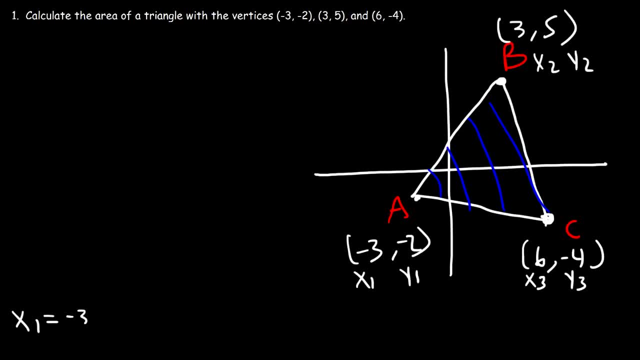 rewrite these values. So X1 is negative 3, Y1 is negative 2.. X2 is 3,, Y2 is 5. And X3 is 6, Y3 is negative, 4.. So I no longer need this picture. just that was for just. 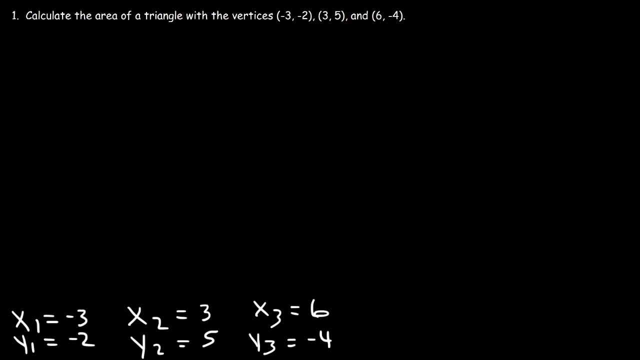 a visual illustration. Now. here's the formula that we need to calculate the area of the triangle. It's 1: 1⁄2, the absolute value of X1, Y2 plus X2, Y3 plus X3, Y1, and then minus. 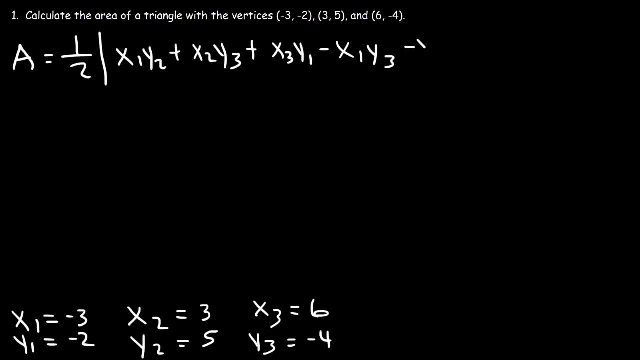 minus and the derivative can be negative. 3,. the Kanal G photo in red is blue, so we can calculate an absolute value of 1, 1⁄2, which is the rotation angle, which will be 0.. blockage all over And plus. 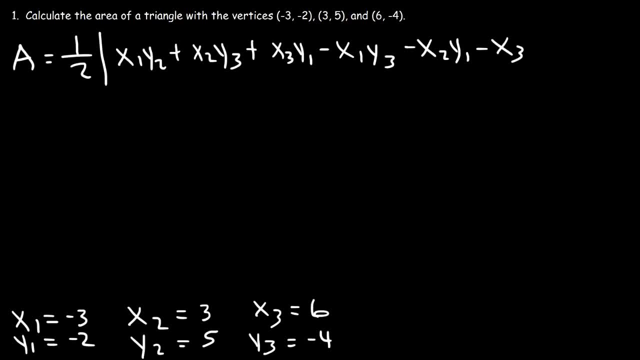 is the the value of x1, x2, plus x3 times 1.. So this is a very detailedesis And I'll minus x3, y2.. So in this example, x1 is negative 3, y2 is 5,. 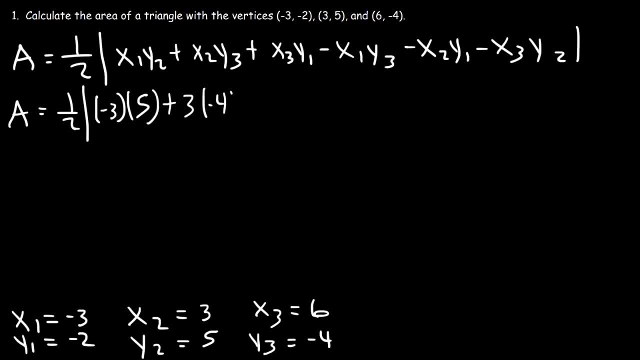 x2 is 3,, y3 is negative 4,, x3 is 6,, y1 is negative 2,, and then minus x1,, which is negative 3,, and y3 is negative 4.. Then minus x2,, which is 3,. 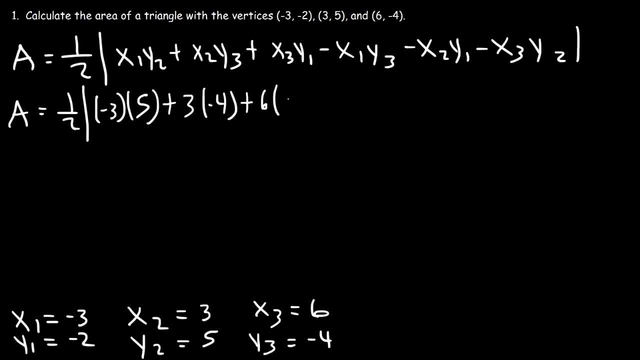 negative 4.. x3 is 6,, y1 is negative 2. And then minus x1,, which is negative 3, and y3 is negative 4.. Then minus x2, which is 3, and y1, that's negative 2.. And then x3 is 6. 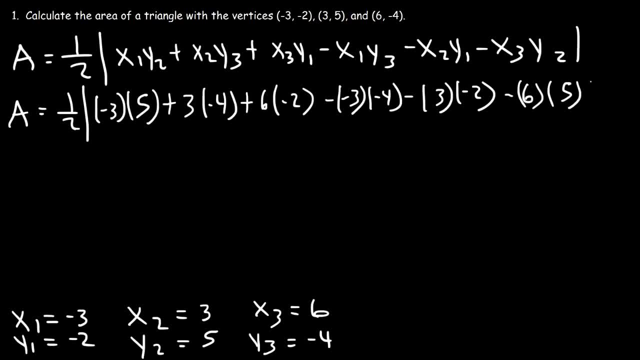 y2 is positive, 5. So negative 3 times 5, that's negative, 15.. 3 times negative: 4 is negative, 12.. 6 times negative: 2 is also negative, 12.. Now negative: 3 times negative: 4 is positive, 12.. 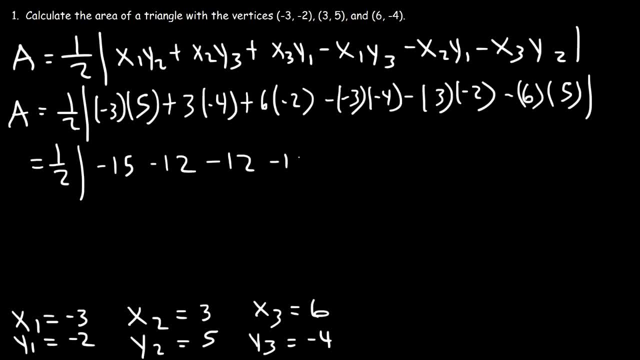 But we do have a negative sign in front of it, so that's going to be negative 12.. And then negative 3 times negative 2, that's positive 6.. And then we have negative 6 times 5, which is negative 30.. Now let's simplify the expression that we now have. 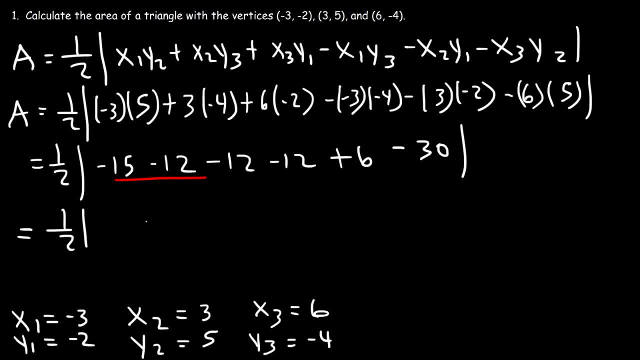 So first negative 15 minus 12, that's negative 27.. And then negative 12 minus 12 is negative 27.. And then we have 6 minus 30, which is also negative 24.. Negative 27 minus 24, that's negative 51.. 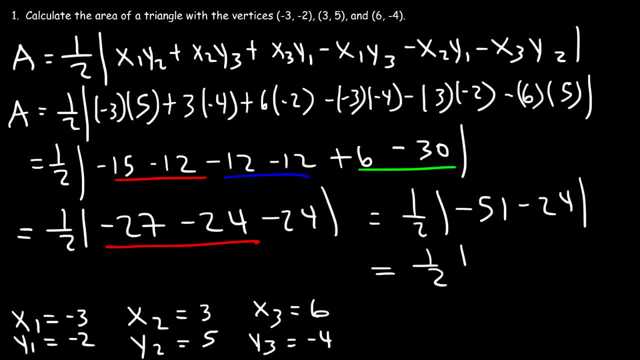 And so negative 51 minus 24, that's negative 75. And the absolute value of negative 75 is positive 75.. So the final answer: you can write it as 75 over 2, or, if you want, the decimal answer, 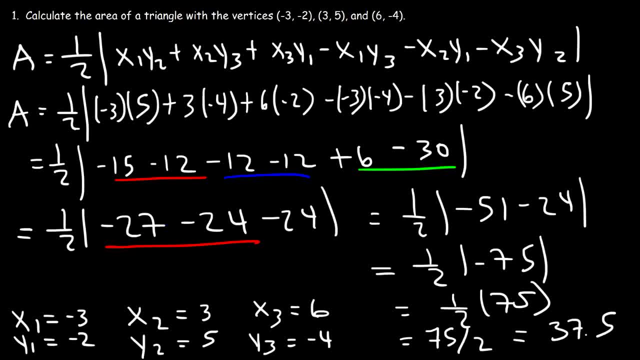 it's 37.5.. So the area of this particular triangle is 37.5 square units. So that's how you can calculate the area of a triangle if you're given the 3 vertices of that triangle. So that concludes this lesson. 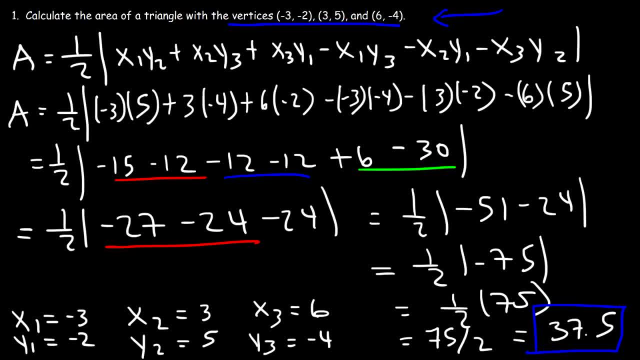 If you want to find more videos on geometry, algebra, trigonometry, calculus and more, or even chemistry and physics- I got topics on those. feel free to visit my channel and just check out the playlist that interests you. I have a lot of topics listed in order. 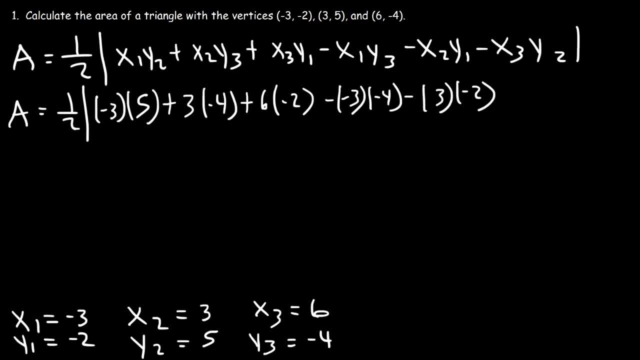 and y1, that's negative, 2.. And then x3 is 6,, y2 is positive 5.. So negative 3 times 5, that's negative 15.. 3 times negative: 4 is negative 12.. 6 times negative: 2 is also negative 12.. 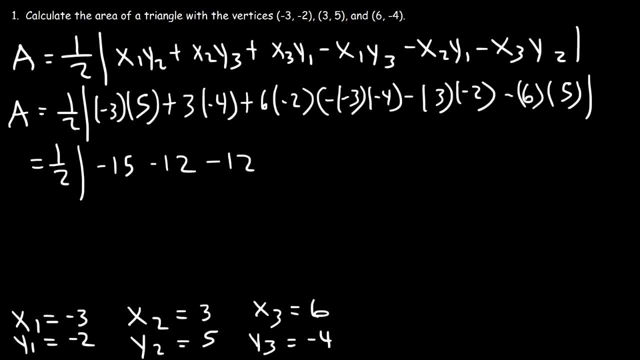 Now negative 3 times negative 4 is positive 12, but we do have a negative sign in front of it, So that's going to be negative 12.. And then negative 3 times negative 2, that's positive 6.. 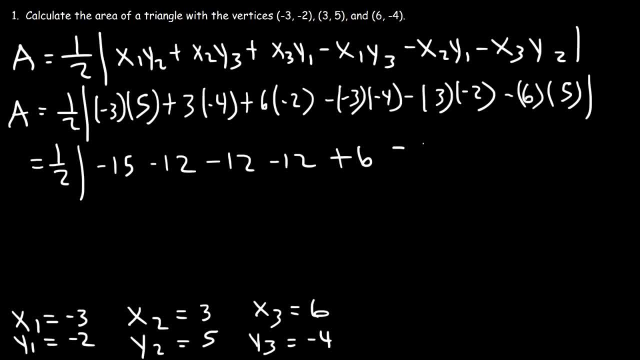 And then we have negative 6 times 5, which is negative 30.. Now let's simplify the expression that we now have. So first negative 15 minus 12.. That's negative 27.. And then negative 12 minus 12 is negative 24.. 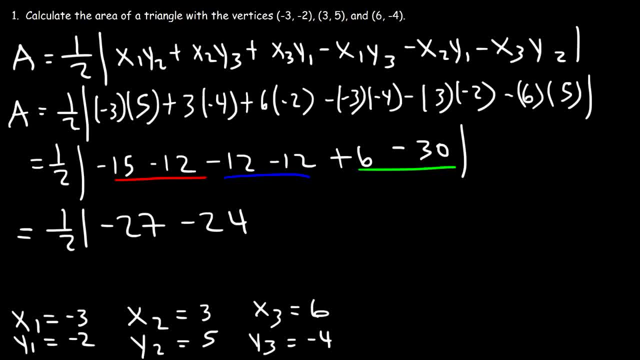 And then we have 6, minus 30,, which is also negative 24.. Negative 27 minus 24,, that's negative 51. And so negative 51 minus 24,, that's negative 75. And the absolute value of negative 75 is positive 75. 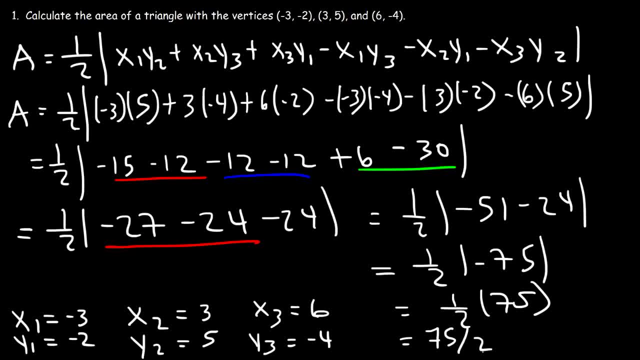 So the final answer, you can write it as 75 over 2, or, if you want the decimal answer, it's 37.5.. So the area of this particular triangle is 37.5 square units. So that's how you can calculate the area of a triangle. 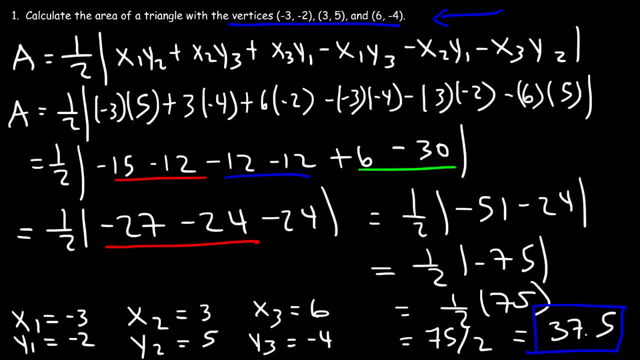 if you're given the three vertices of that triangle. So that concludes this lesson. If you want to find more videos on geometry, algebra, trigonometry, calculus or even chemistry and physics- I got topics on those- Feel free to visit my YouTube channel and I'll see you next time. 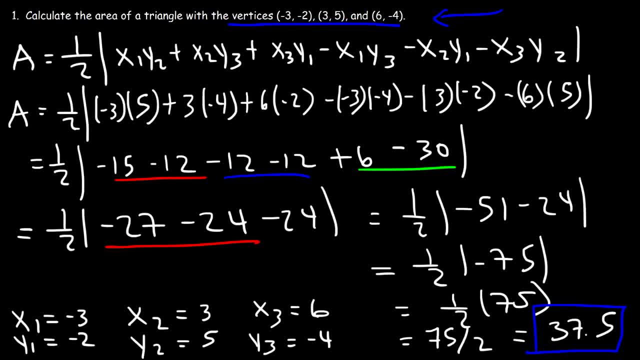 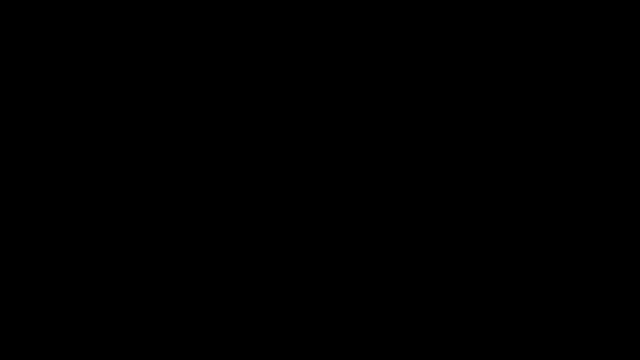 Subtitles by the Amaraorg community. Thank you.